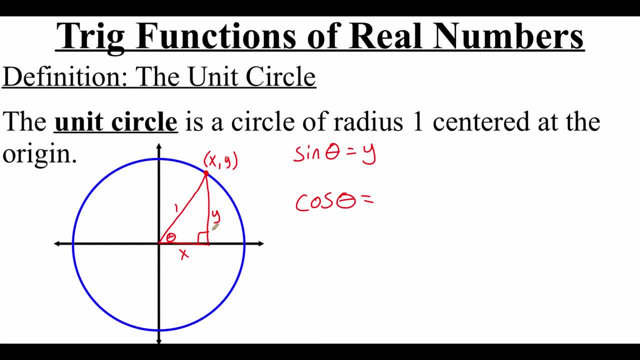 of theta Cosine would be the adjacent side over the hypotenuse. But again, since we're dividing by one, that doesn't change anything. So the cosine is just our x value from the ordered pair. Now, as far as the tangent goes, the tangent of theta, that's still going to be opposite. 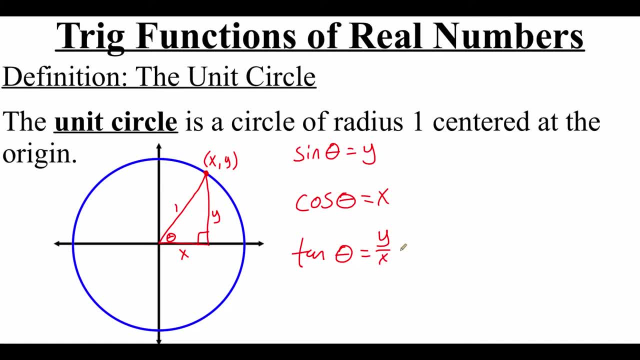 over adjacent, So that's going to be y over x. And we do need to make sure that in the, in this case, our x value is not zero, because we can't have zero on the bottom of the fraction. Now we can also look at those reciprocal functions as well, So the cosecant of theta. 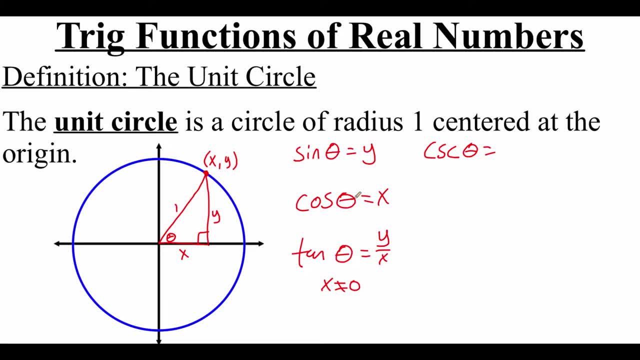 Well, if I flip this over, cosecant would be the hypotenuse over the opposite, So this would be one over the y value. as long as y isn't zero For the secant of theta, that's the reciprocal of the cosines. That would be hypotenuse over adjacent. So that's going to 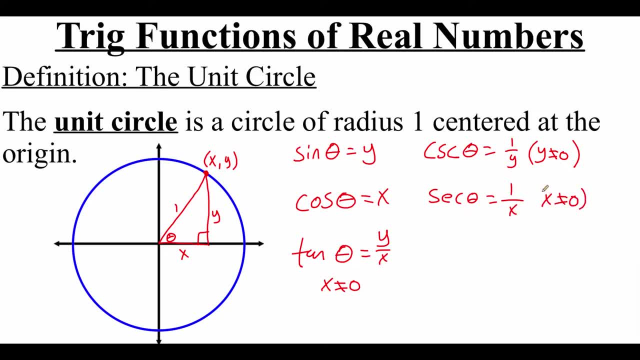 be one over x, And again x cannot be zero. And lastly, the cotangent of our angle theta is going to be the adjacent side over the opposite side, So that's going to be x over y, And in this case y cannot be zero, since we don't want zero on the bottom of that fraction. 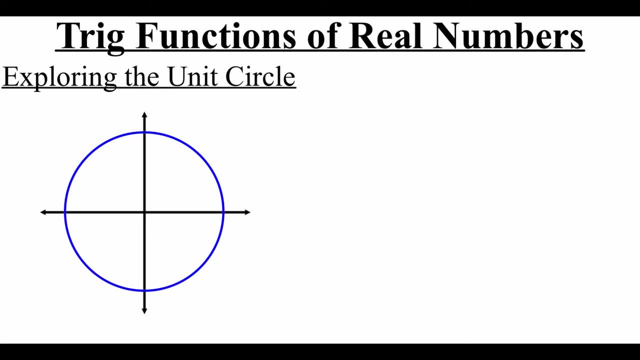 Now we're going to take a look at some general properties of the unit circle And remember the unit circle has a radius with a length of one. So if we start in the middle and go out to the edge of our circle along the x-axis, and that length should be a distance of one, 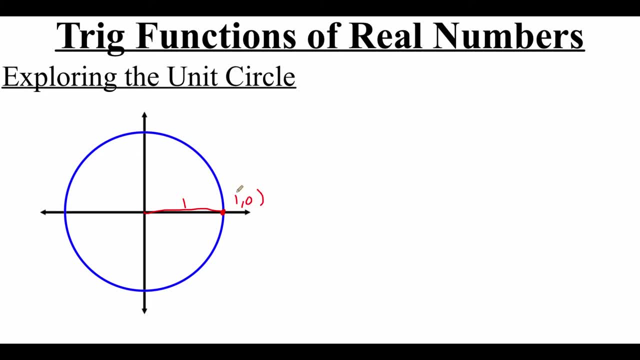 So this point on the circle is going to be the point one- zero. And if we go the other direction a distance of one, then this point on the left-hand side of our circle, since we're going left into the negatives, that's going to be the point negative one- zero. Now, if we focus on those, 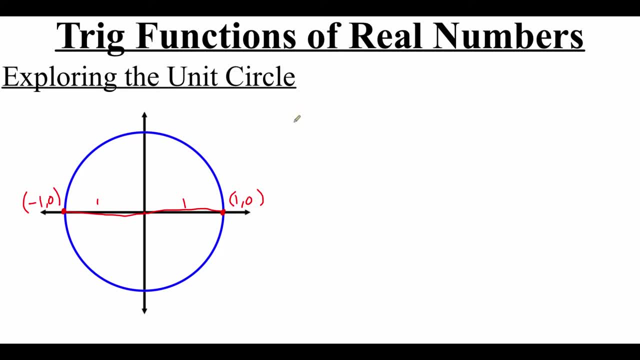 x values. remember the cosine is related to the x value. So because the biggest x value we're seeing is negative one, then our cosine has to be some value between negative one and positive one. Now, if we look at something similar but vertical instead, if we start in the middle and go up, 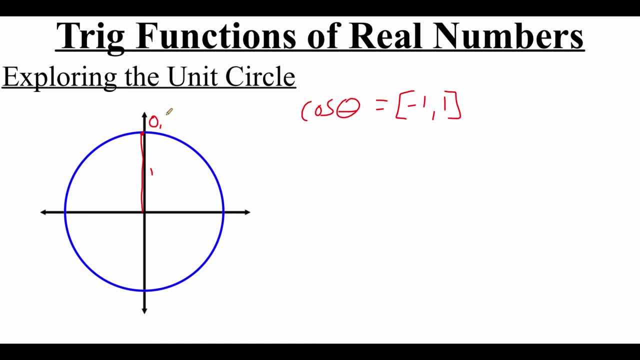 to our circle. again, that's a length of one. So this is going to be the point zero one. And if we do the same thing, going down that length of one, well, we went down, so that means that's a negative one. So this is going to be the point zero: negative one. 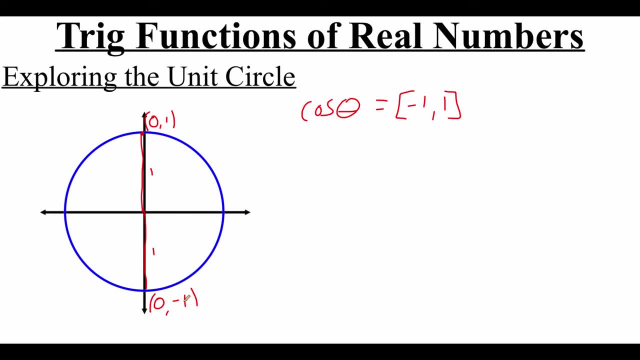 And as we look at the y values, we've got one and negative one. Sine deals with the y values, so our y values for the sine are also between negative one and positive one. Now let's say we had an angle drawn out in standard position, So we're starting along. 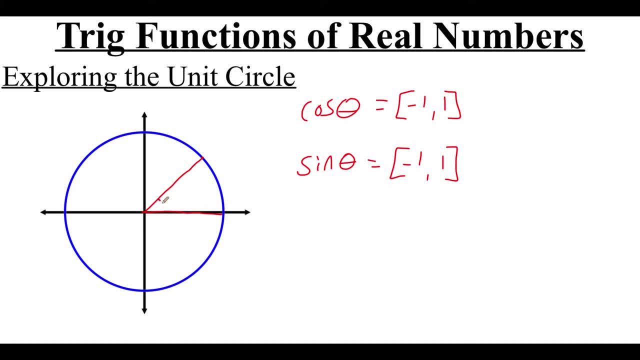 that positive x-axis and let's say we rotate up And this is just going to be some general angle theta and it's going to intercept some point x, comma, y. Now, if we looked at a similar angle but going in the negative direction, so if I went down theta, 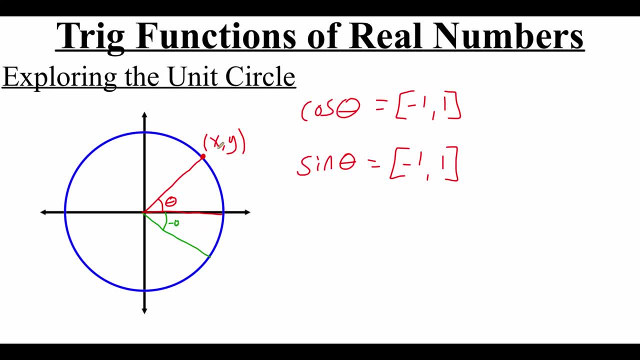 so this angle would be negative theta. Now, what's going to end up happening in here is these ordered pairs are going to be very, very similar to each other, But since we went down, that means the y value is going to be negative. So this is going to be x and negative y. Now notice that these x. 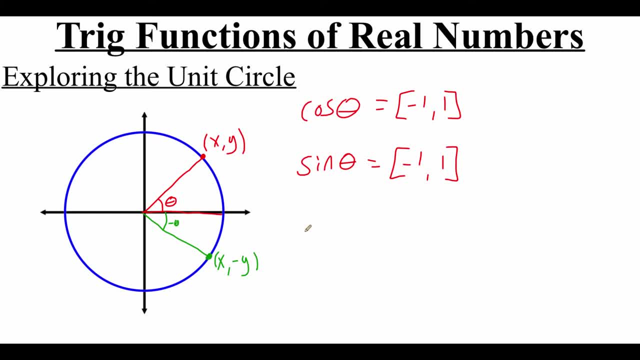 values are exactly the same And remember, x values deal with the cosine. So we can say that the cosine of theta is equal to negative y And if we look at the y-axis, we can see that the y-axis is equal to the cosine of negative theta, since those have the exact same x value in their ordered. 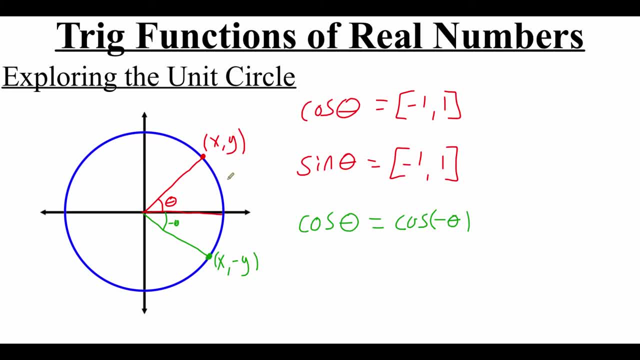 pair. Now if we want to look at the y values, those are opposites of each other. So what we can say in here is that the sine of negative theta is equal to the opposite of the sine of theta. Now let's look at some general x and y ordered pair out on the edge of our circle. Now what I 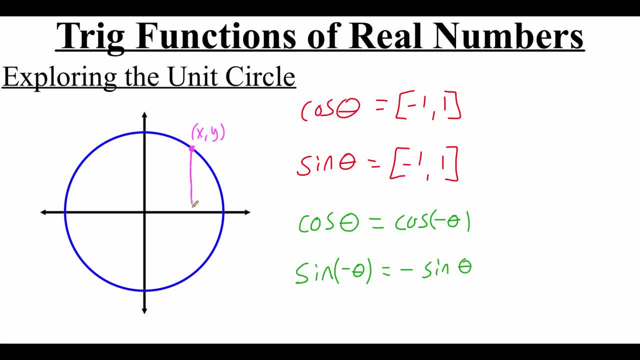 can do with this is: I can actually form a right triangle. I can drop down a vertical side from that point and then I can connect that to the origin, and then I will connect the origin directly to that x and y point, So that forms a right triangle in here. Now this x value tells us the 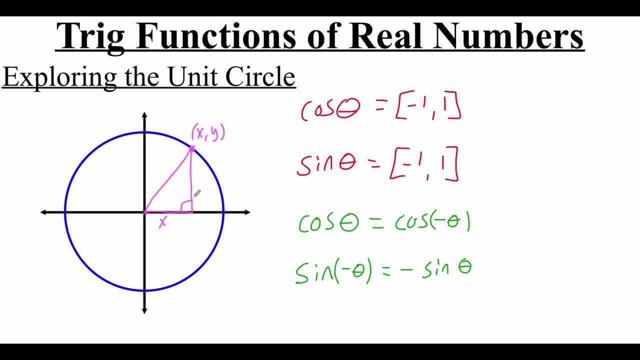 distance horizontally away from the origin, and this y value tells us the distance vertically from the origin. And then this hypotenuse: since we're dealing with a unit circle, that length is just one, because that's the radius of our circle. Now we know that the y value is equal to the